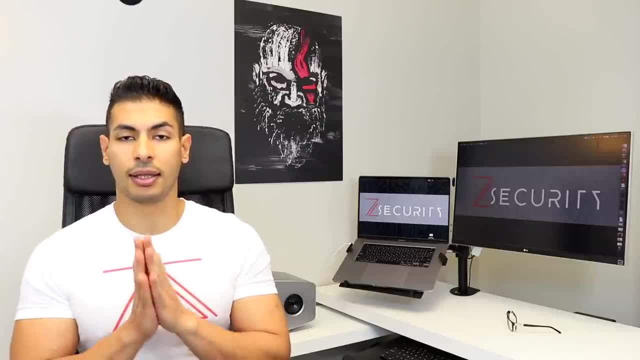 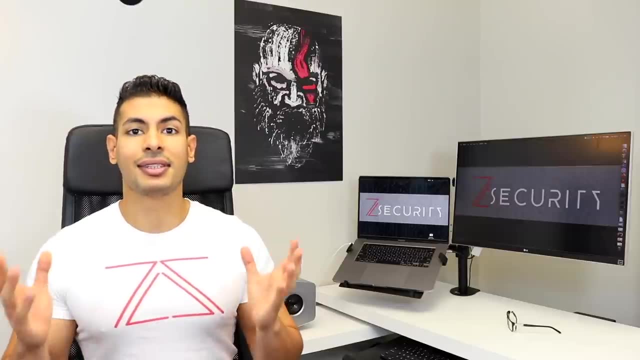 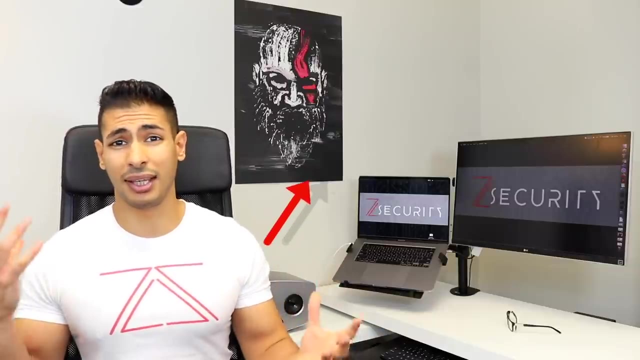 the most important points that you want to keep in mind and the most important things that you need to learn in order to protect your privacy and anonymity. now, this is a huge topic. it is impossible for me to cover it in one video. i actually have a full course, which is about 11 hours of content to teach. 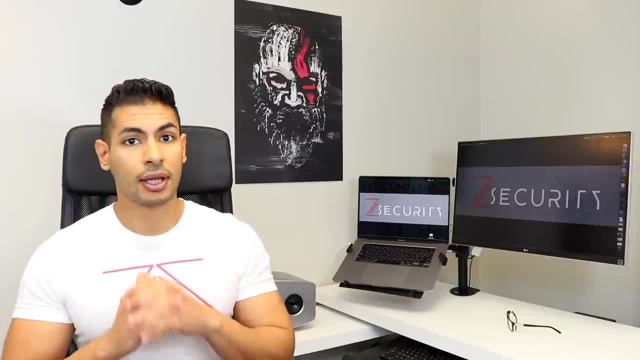 you how to protect your privacy, anonymity and access the dark web, so i'm gonna go through the main points in this video. if you don't understand anything or you feel like you need to learn more about privacy and anonymity, then go ahead and check out the next video. i'll be showing you how to. 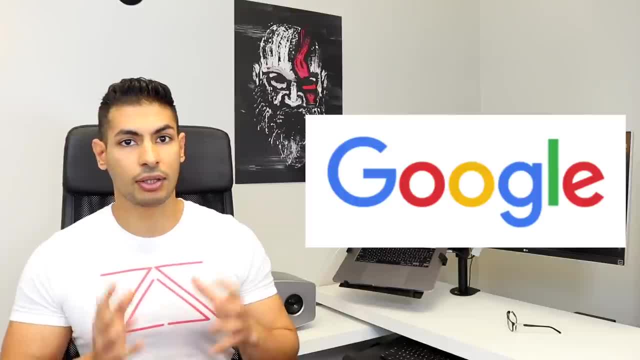 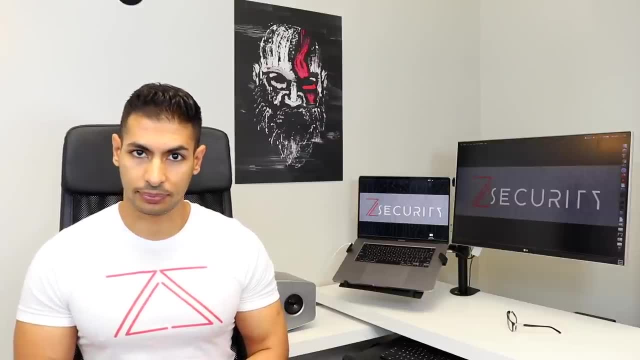 about a specific point, then google is your best friend. go ahead and do some research on it or, if you want, you can get my course if you don't want to spend time researching. so, first of all, the main thing that you want to do is make sure that your connection to the internet 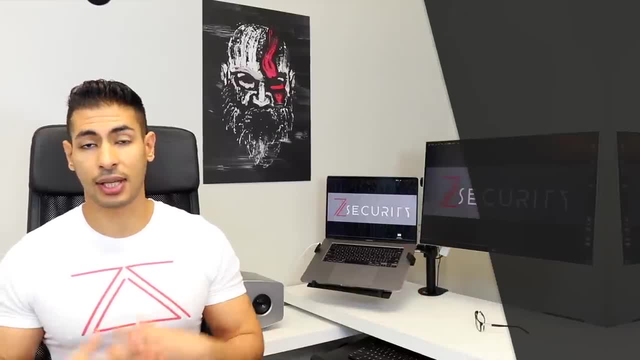 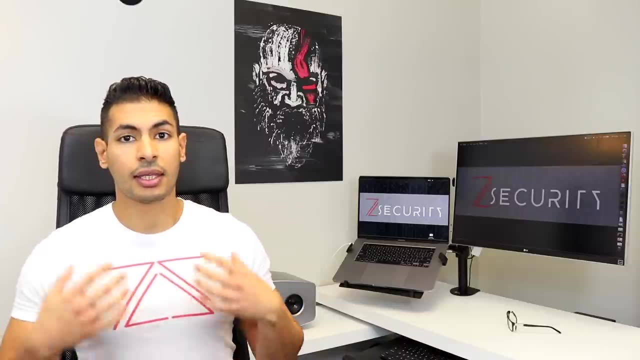 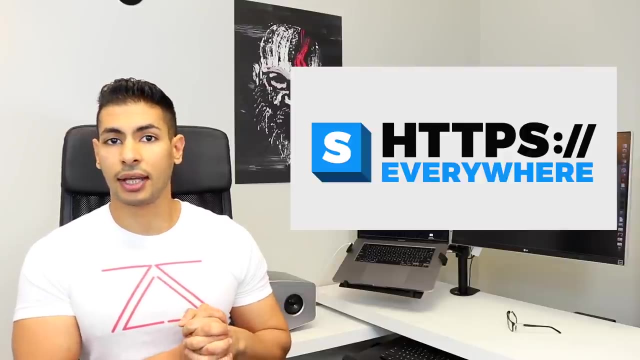 is private. so, like i said, when you access any websites or do anything on the internet, you want to make sure that the data that you send and receive is private. doing that is simple enough. you can simply use a plugin such as https everywhere. this will make sure that all the 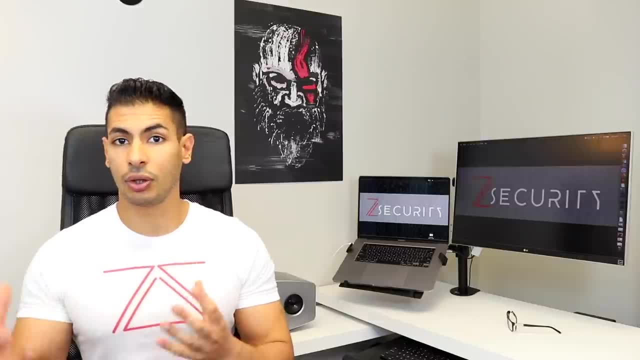 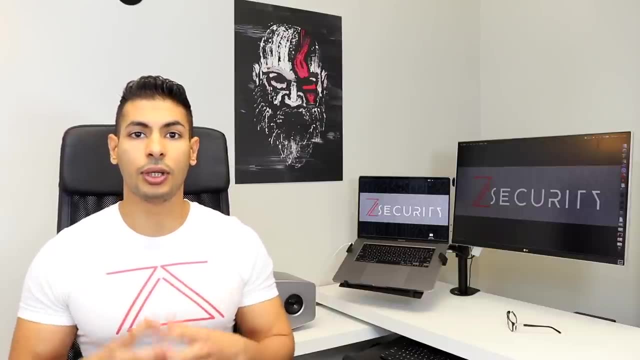 connections are done over https, which means that all of your data is going to be encrypted. therefore, even though it's going to pass through a number of hops, and even though we know that it is possible for government entities and for hackers to intercept these connections, they will be able to read our data, but our data is going to be encrypted. it's going to be gibberish. 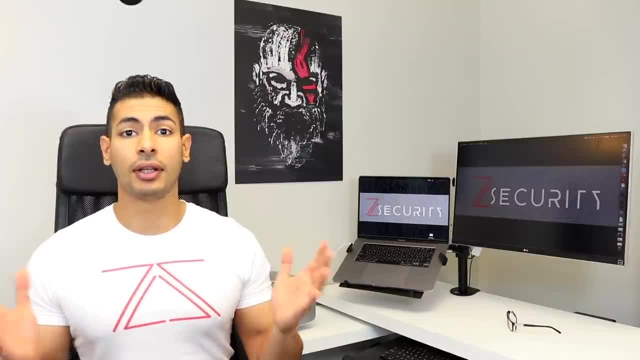 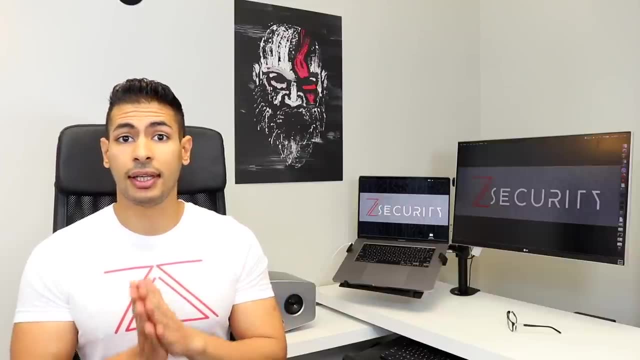 they will be able to read our data, but our data is going to be encrypted. it's going to be gibberish. therefore, it's going to be useless to them. now, this will ensure that your connection is private, but you're still not anonymous. the servers and the websites that you communicate with 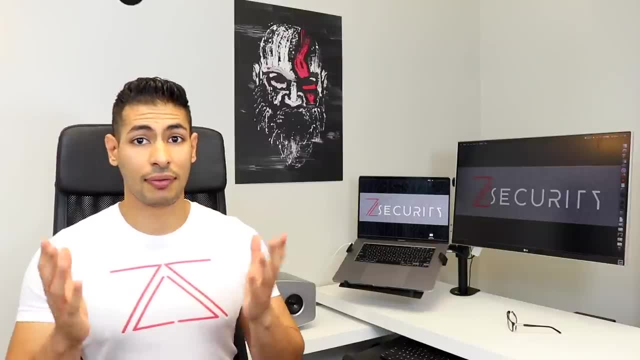 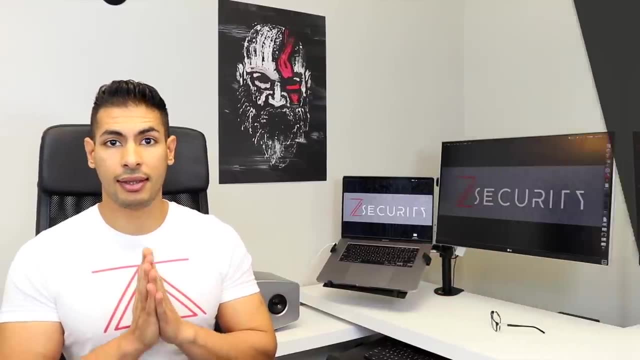 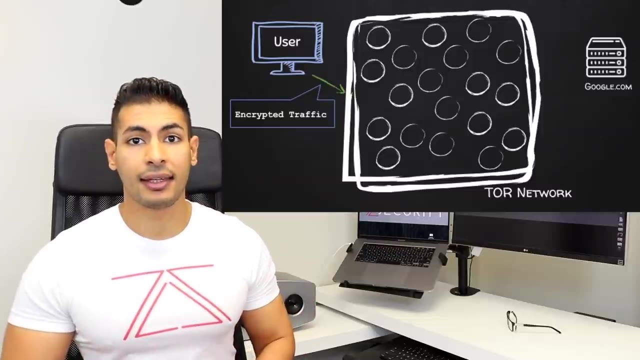 will still be able to see your location. so if you want to protect your anonymity, then you should use an anonymizing network. a very popular one is the tor network or the onion router. tor works by first of all encrypting your traffic and then it randomly selects. 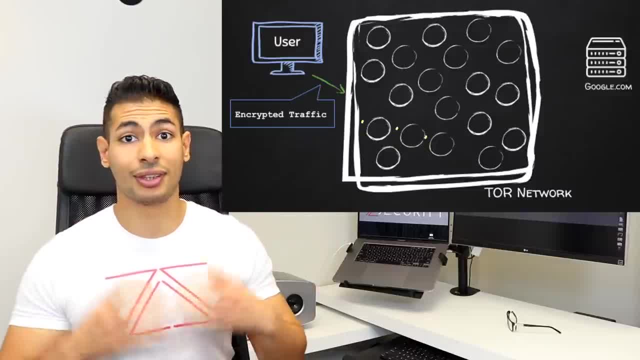 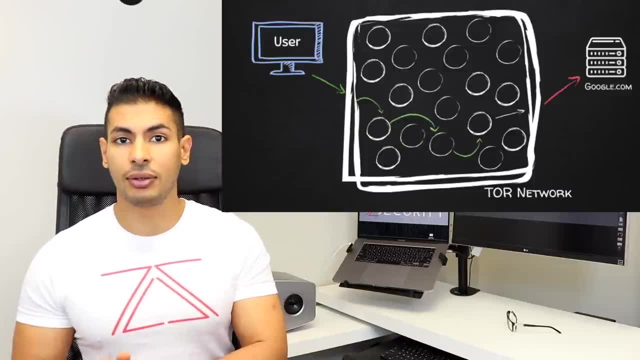 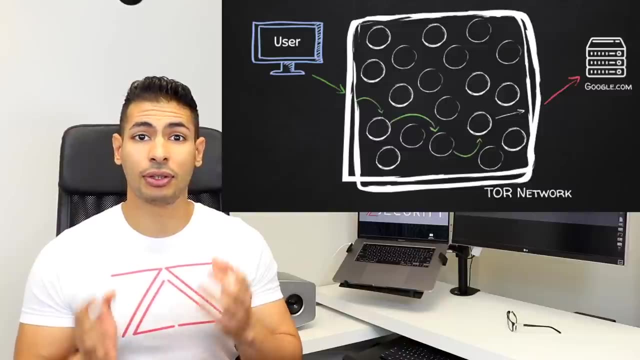 three nodes or three computers out of the network, which contains a lot of computers, and then it first passes your data through these three nodes before sending it to the destination. now the tor network is free and open for everybody. therefore, at any point of time, lots of people might be using this network and lots of people might be using the three. nodes that you are using. therefore, even if someone manages to compromise this network and analyze what's happening in it, it would be very difficult to separate what you do from the traffic generated by all of the other people that are using the same three nodes. you can also use a vpn, so the vpn again will first add another layer of encryption to your data. 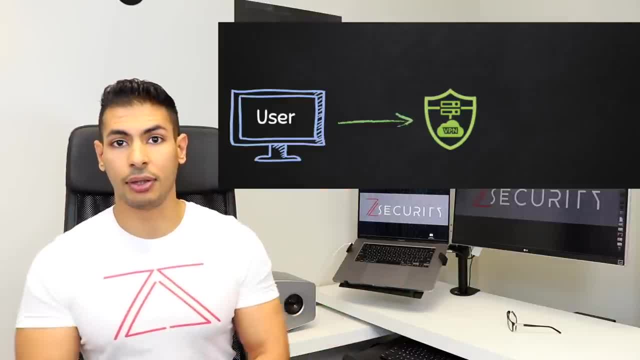 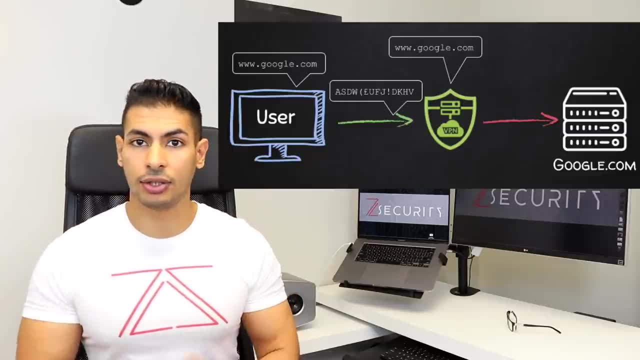 and it will send it to a middle server that could be anywhere in the world, and then from there, your data will go to the destination again. this adds another layer of encryption and hides your identity, and you can even use tor and a vpn at the same time for extra protection. 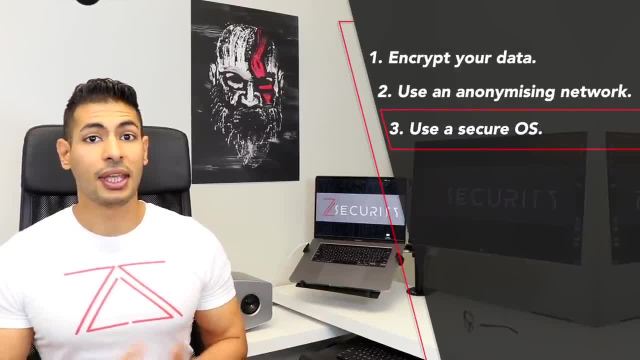 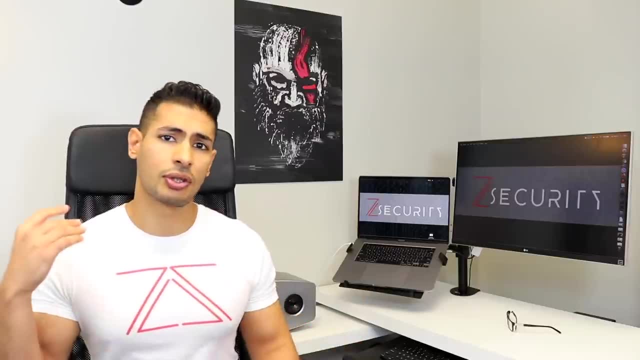 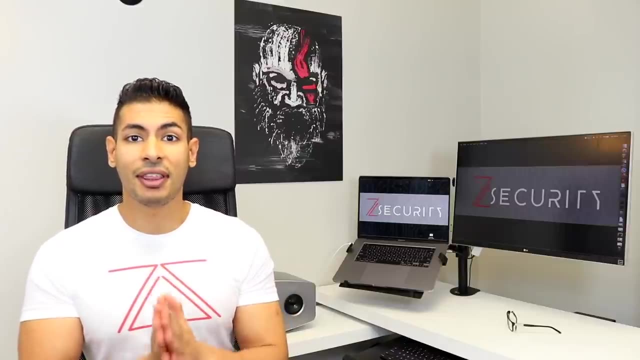 last but not least is security. so even if you're using a great anonymizing network, you're bouncing your traffic through a number of servers and you're using all sorts of encryption to protect your privacy, if somebody manages to gain access to your computer, everything you're doing is useless because they can de-anonymize you. 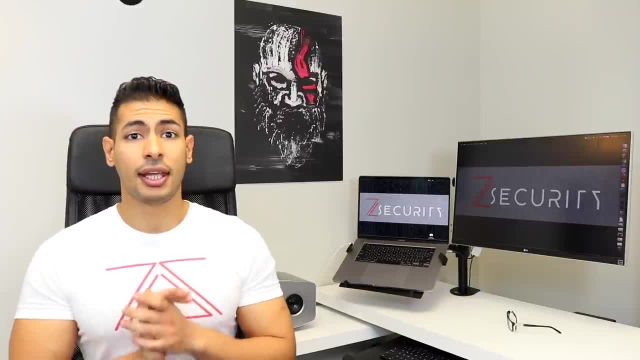 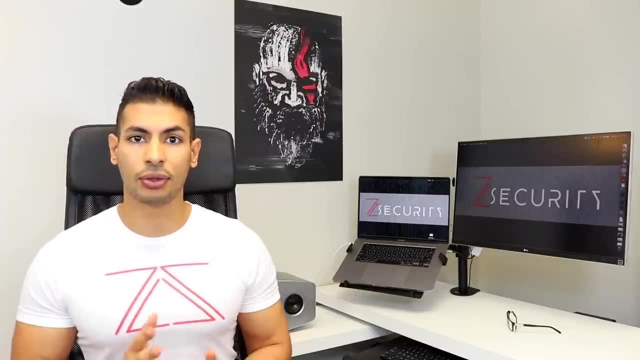 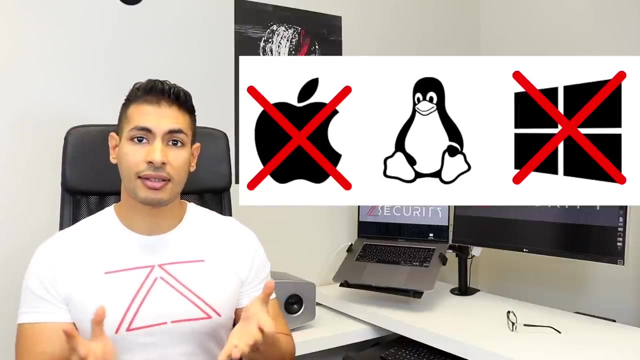 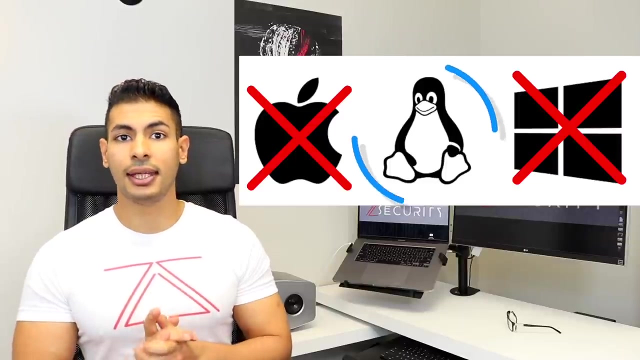 very easily. therefore, if you're serious about protecting your privacy and anonymity, it's very important that you use a secure operating system, so you should really consider moving away from windows and osx. these operating systems are not very secure and they also log a lot of data about you anyway. linux would be a great option that balances between security, privacy. 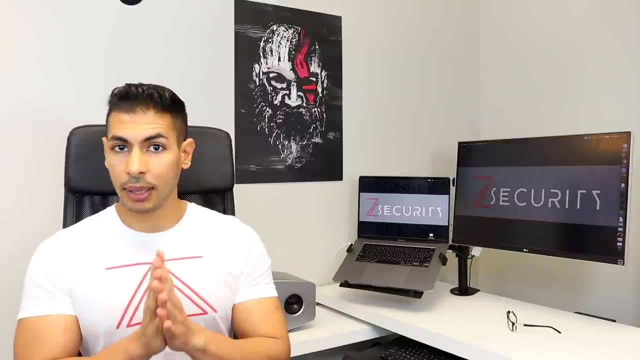 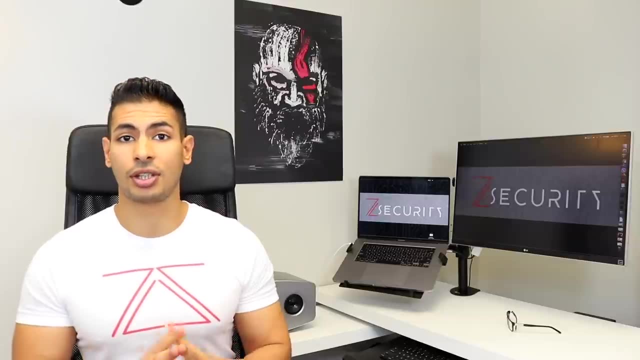 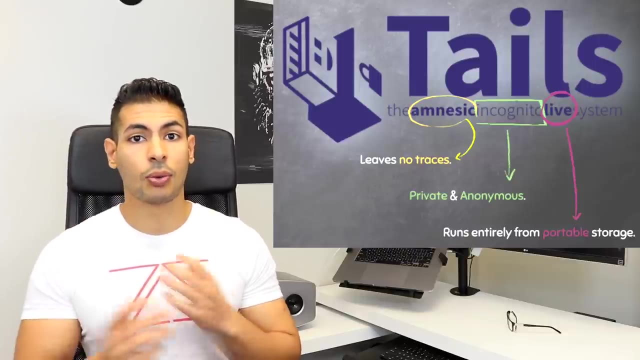 and ease of use, but if you really want to protect your privacy and anonymity, consider using an operating system that is designed for that purpose, such as tails os. this is a live and amnesic operating system that you can boot from a usb stick. once you reboot, it removes everything. it routes all. 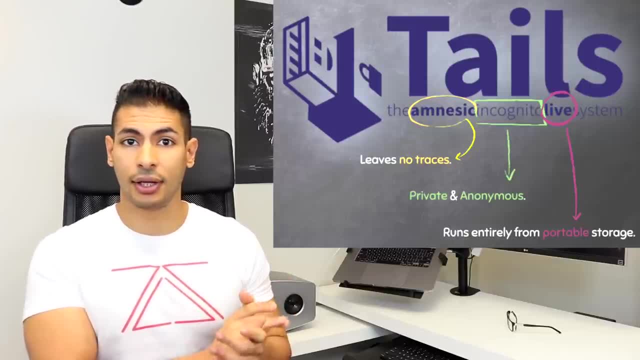 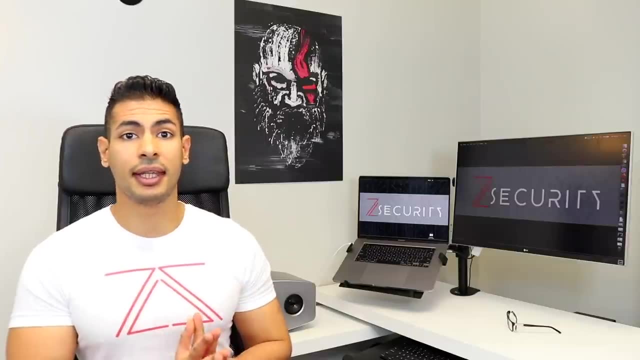 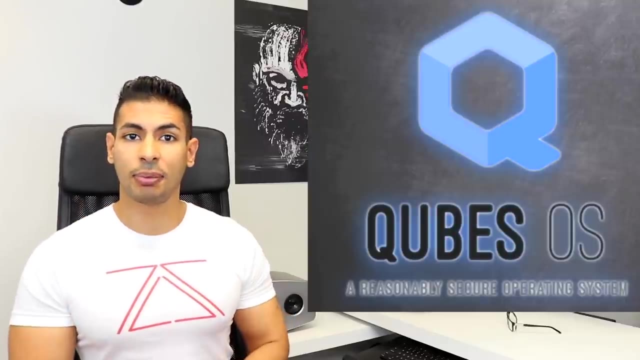 traffic through the tor network to protect your privacy and anonymity, and it actually comes with a lot of really useful privacy tools. if you really want to take your security to the next level, then i highly recommend looking up cubes os. this is an amazing operating system that is designed from the ground up to be very, very secure. it separates everything into different 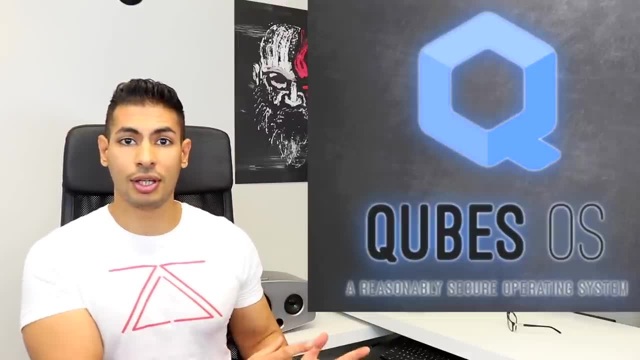 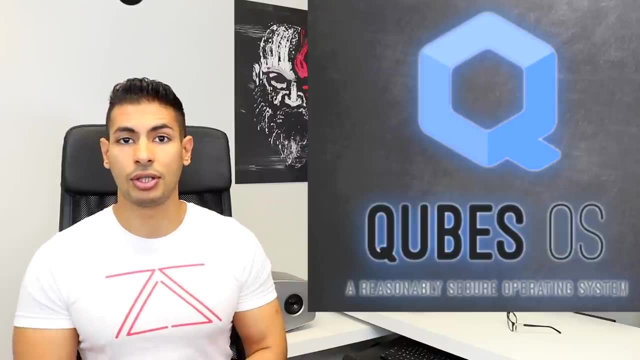 domains and everything runs into separate virtual machines that cannot really interfere with each other. it has really cool features, such as disposable virtual machines to run suspicious files, volt machines to store sensitive files, hoonix gateway to route all traffic through the tor network and so much more. you should also always 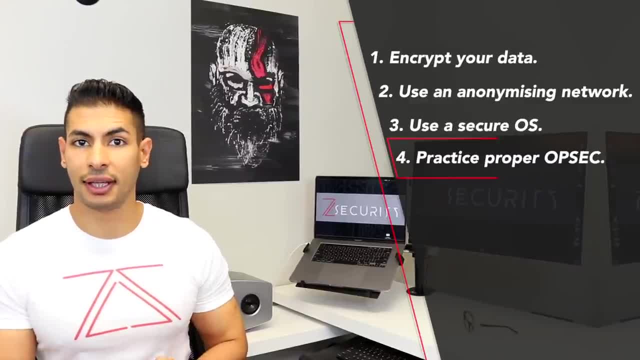 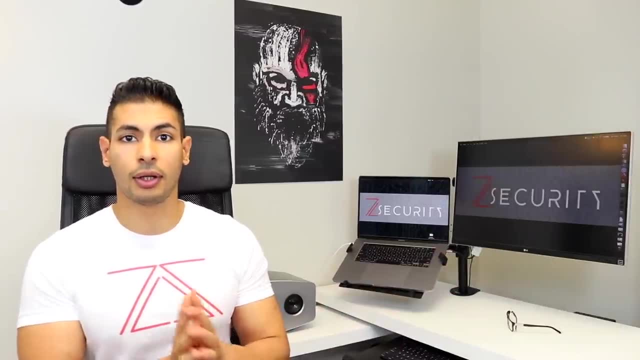 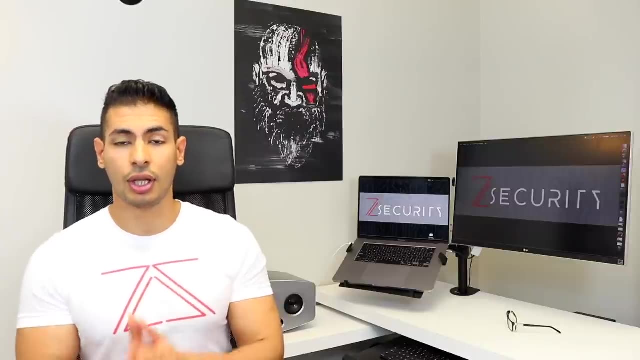 be aware and smart with what you do on the internet. so it doesn't make sense that you follow everything that i said so far and then you go and log into your gmail or facebook account that already contains all of your information, your friends and the previous locations that you used. 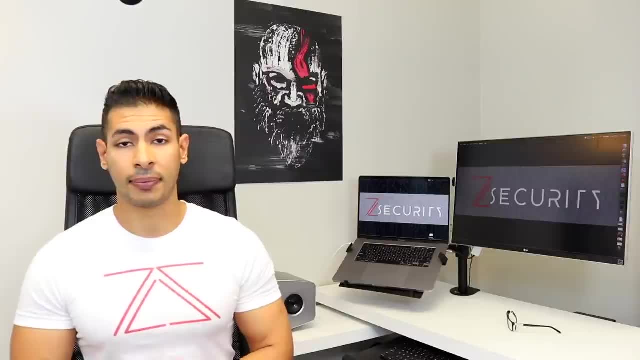 to log into these accounts. that will jeopardize everything. so you want to be smart with this. so you want to be smart with the services that you use, from your email services to instant messaging, to search engines- pretty much everything you do on the internet. you need to think twice about it. 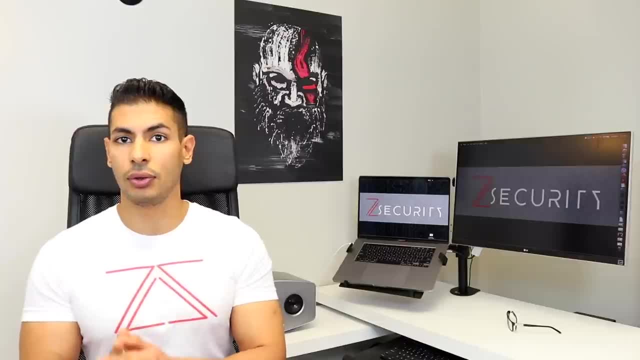 and try to move to more privacy focused solutions. for example, instead of using gmail, use protonmail or even use a dark web email provider that is more private and more secure. i'm only using gmail here as an example, but this goes for all of the services that you usually use on the internet. 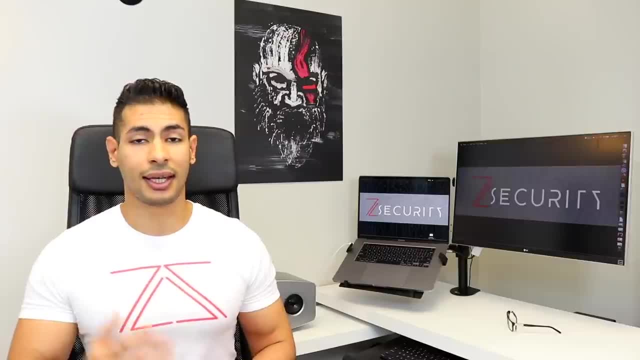 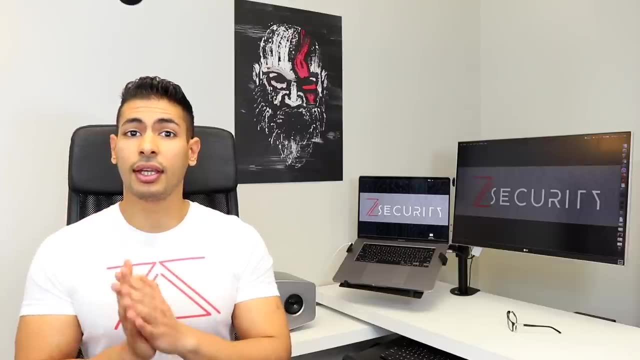 so, like i said, from instant messaging to downloading and uploading, and even social networks, you want to be very smart with what you do, and you should also think twice about the information that you share on the internet. think about the people that you communicate with, the way you type your emails. all of these things can be used as clues and pieced together in order. 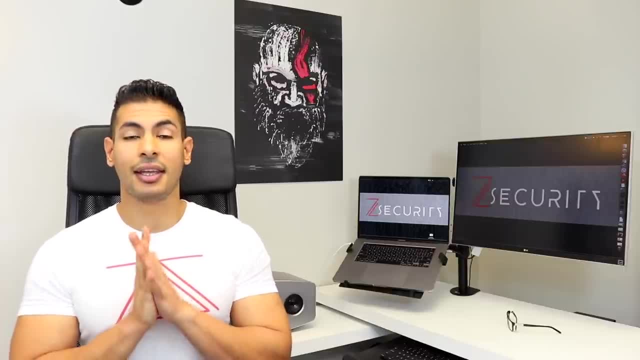 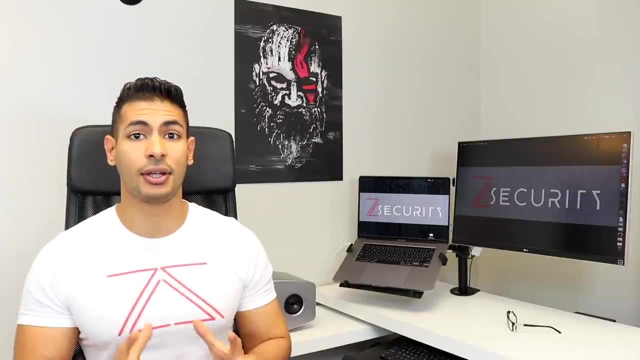 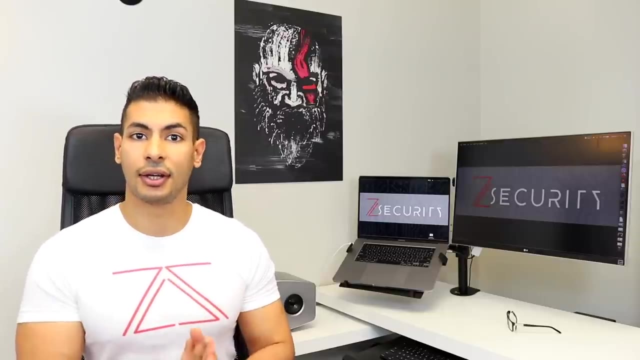 to de-anonymize you. like i said, it is impossible to be a hundred percent sure that you are not 100 invisible. all we're trying to do is protect our privacy and anonymity as much as possible and make it as difficult as possible for others to track us and de-anonymize us. it's simply a matter. 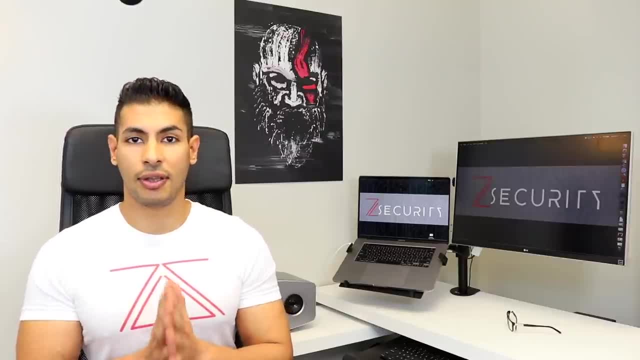 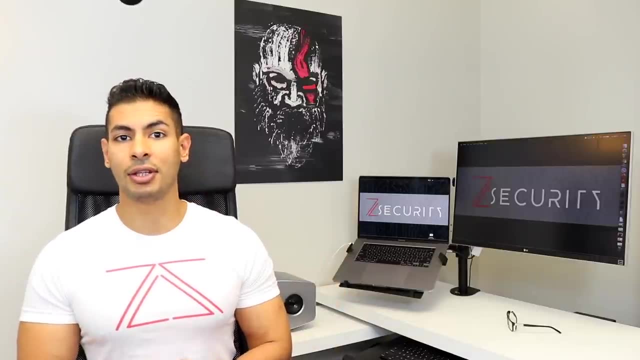 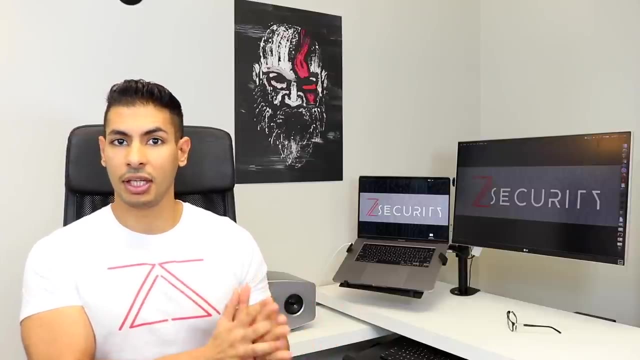 of how much time, money and effort they want to invest into tracking you and de-anonymizing you. now, i hope i didn't miss anything major. these are the main points that you want to look for, in my opinion. like i said you, you google to learn more about any of these points. i'm sorry i couldn't dive too deep into any of them.